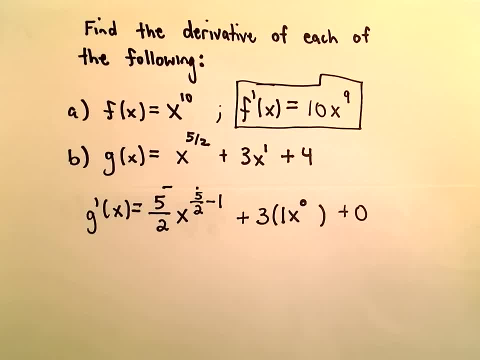 The derivative of a constant is just 0.. So the plus 4, normally we don't write plus 0, but I'll write it here just to be, you know, kind of hopefully clear about what's going on. All right, well, so we've got 5 over 2 times x to the 5 halves. 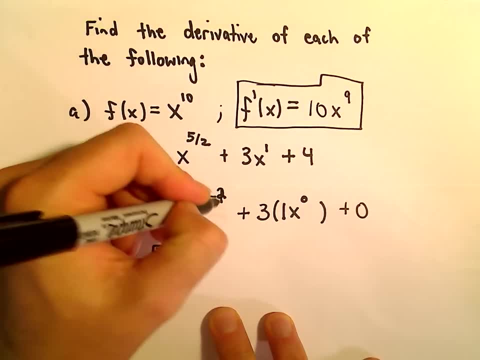 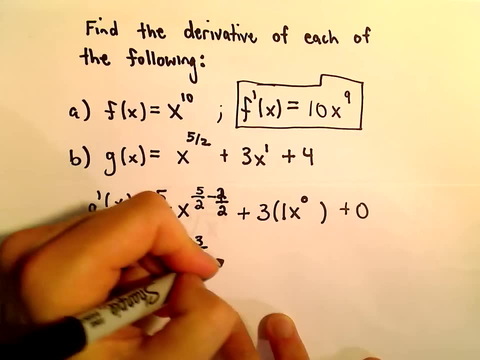 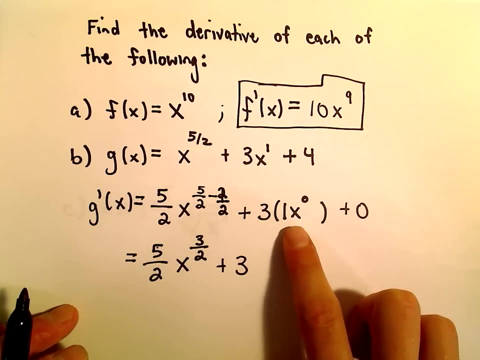 Well, we would have to get common denominators. So instead of minus 1, we could write that as 2 over 2.. Well, 5 minus 2 will give us 3.. 3 over 2.. When we take a number and raise it to the 0 power, we're going to get just 1.. 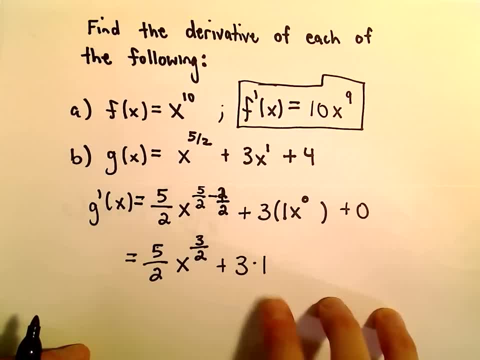 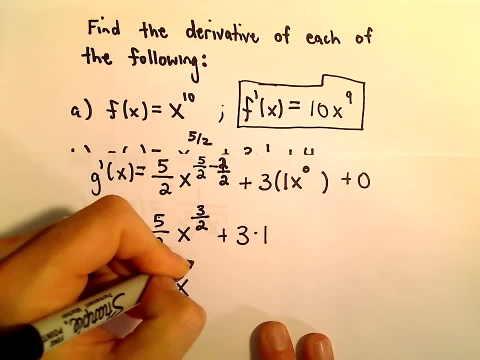 So we can just write: 3 times x to the 0 is 3 times 1.. Again, the plus 0, we'll leave it off. So it says our derivative is going to be 5 halves times x, raised to the 3 over 2 plus 3.. 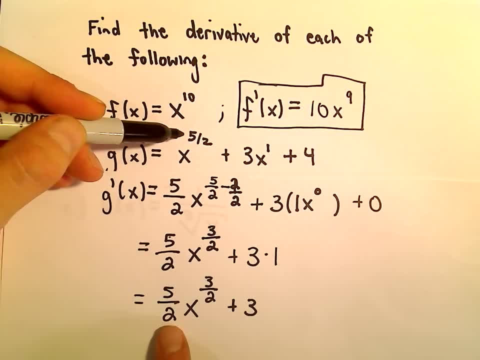 So what happens is again, you know, the 5 over 2 just comes out front like normal. You know, hey, it's a fraction, but if you subtract 1, you're just subtracting 2 over 2 in this case, which gives us 3 halves. 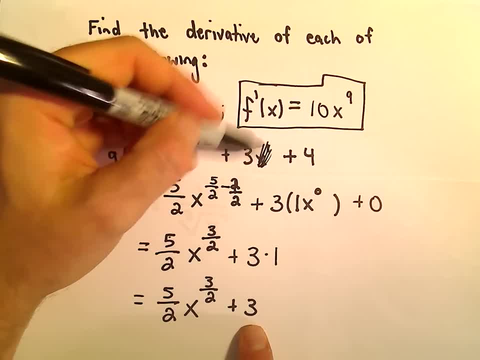 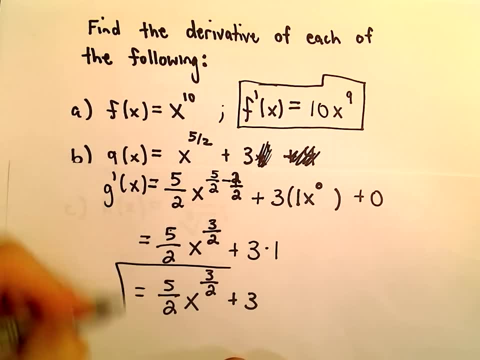 When you have a number times a variable to the first. basically the variable just goes away when you take the derivative And then the constant just goes to 0.. So that would be our derivative for part B. And last but not least, let's look at our last one here. 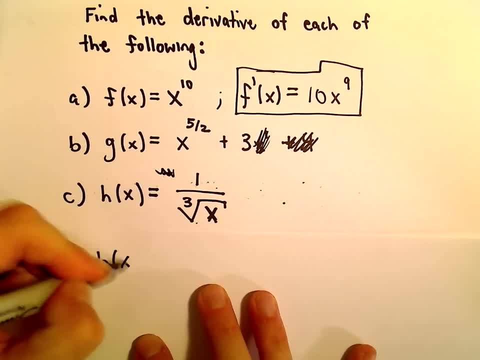 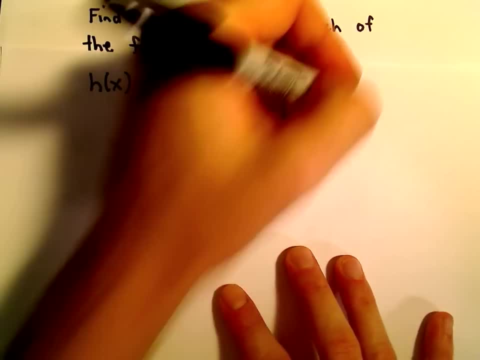 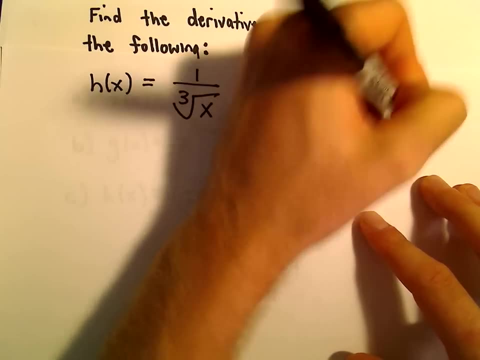 So we've got. so we had h of x equals 1 over the cube derivative. So that's the root of x And maybe just to remind you, remember the. so if we have x raised to the m and then the nth root of that, we can write that as x raised to the m over n. 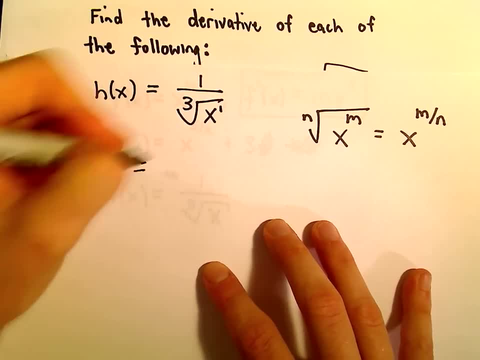 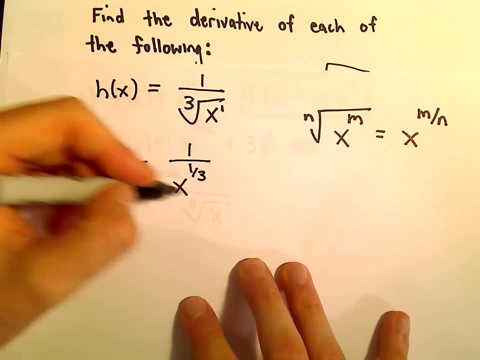 So you can think about this as being x to the first power underneath, So we could really rewrite this as 1 over x raised to the 1 third power. Well, to use that derivative rule, we need sort of the x to be in the numerator. 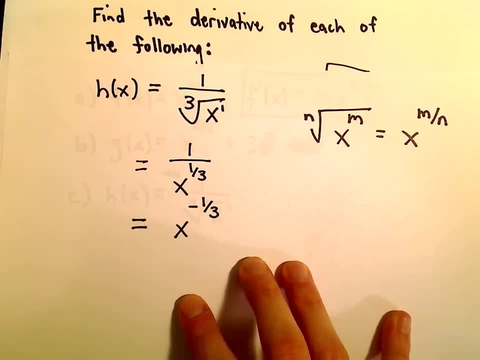 Well, I can pull the x upstairs And I just have to try to get it to the right. So I'm going to change the sign on the exponent. So, really, h of x. I can rewrite that as just saying it's x to the negative 1 third.